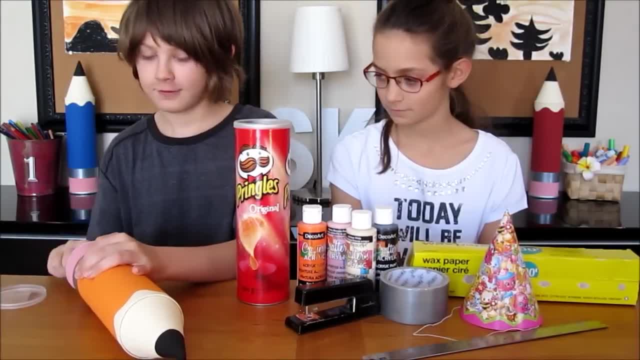 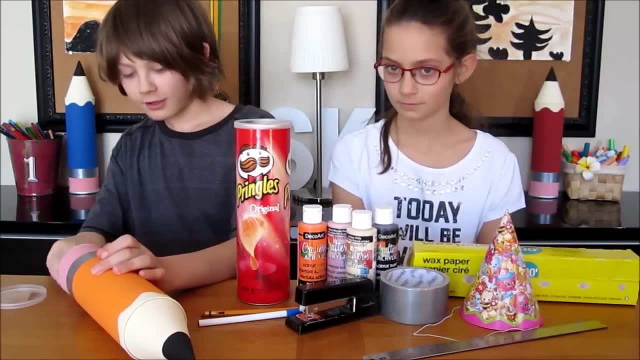 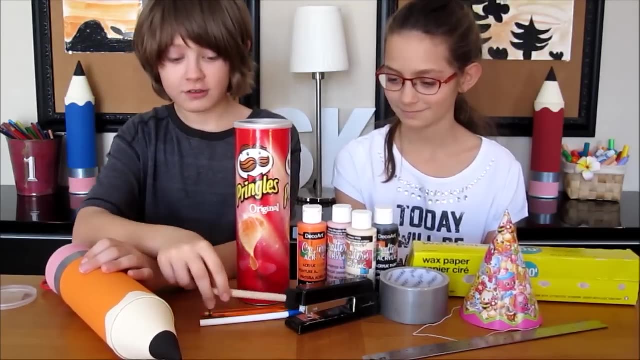 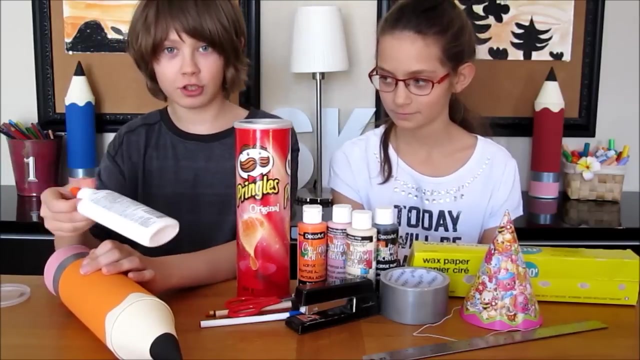 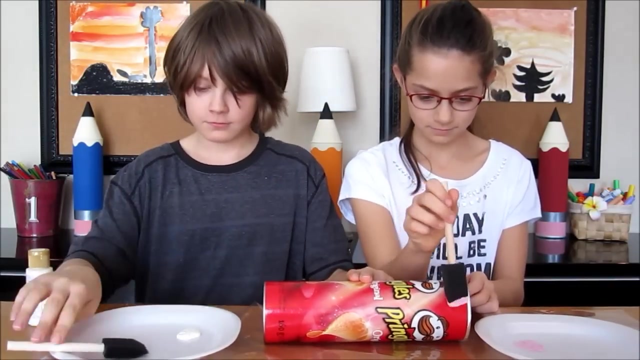 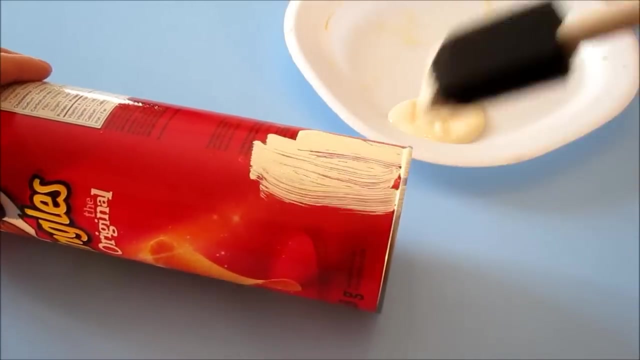 also need a pen, a pencil, a paint brush, a foam brush, scissors and some glue. To make this pencil case, we need a thick and thick sheet of cardboard, a pencil and paper towel and a piece of paper. We're going to need a paper towel and a pencil. Then we 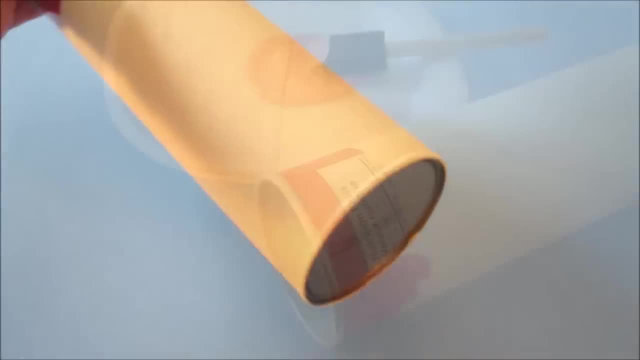 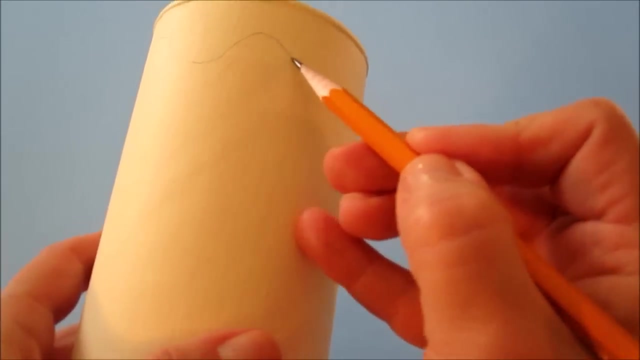 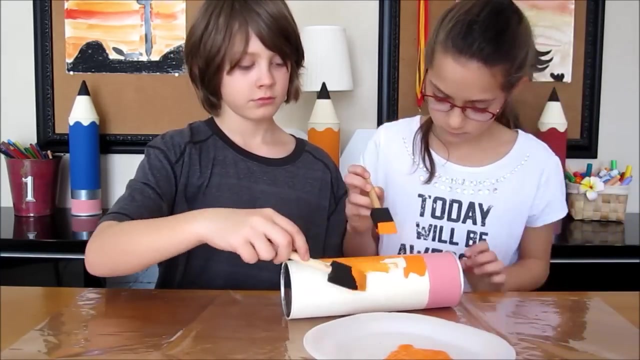 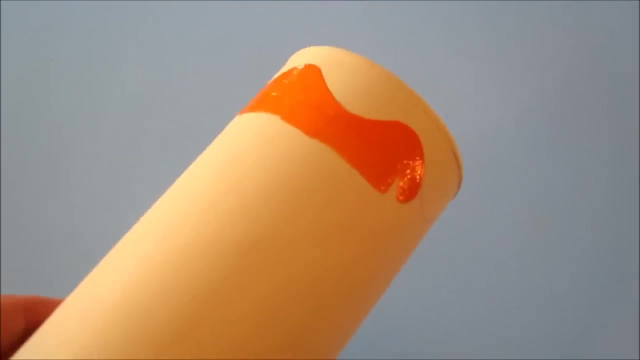 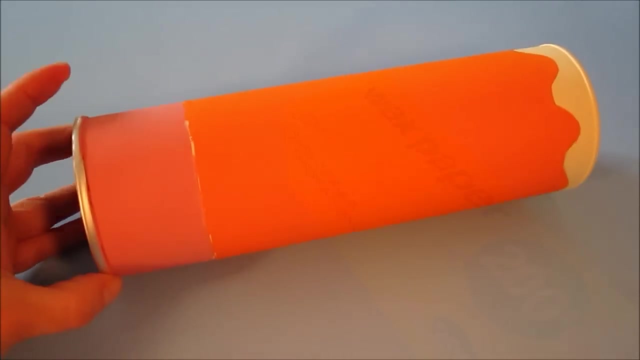 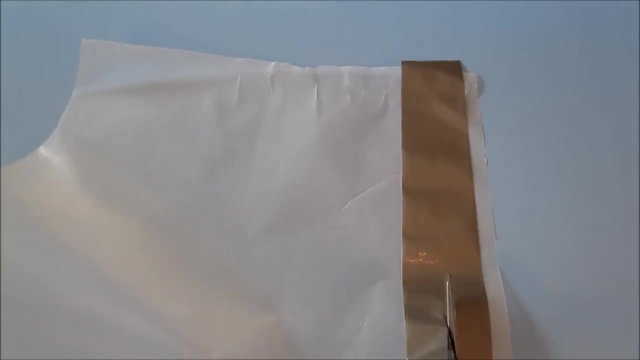 take a piece of paper and a rubber band, Then we put it on the back and open it, Then use a rubber band to roll it up, Then lay the paper on a paper towel, Then slide the paper back in the box. Thank you, 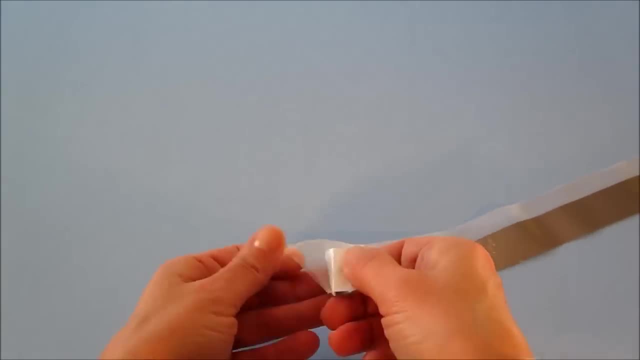 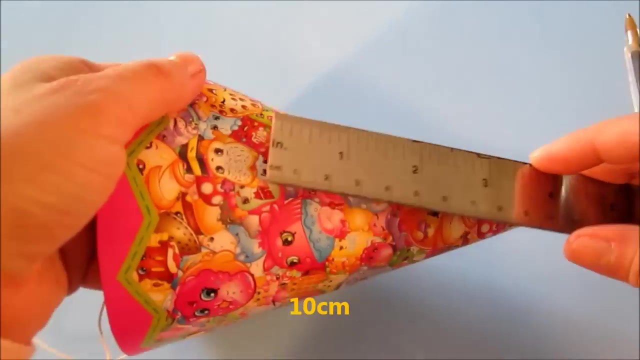 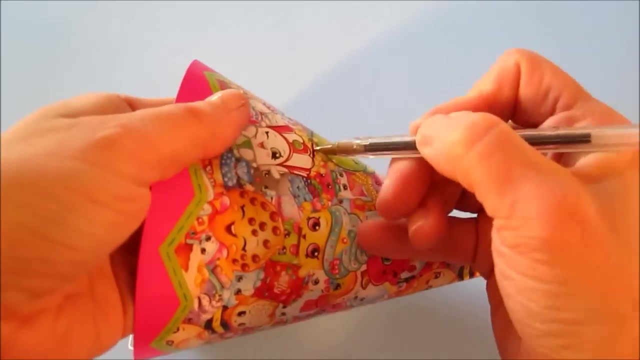 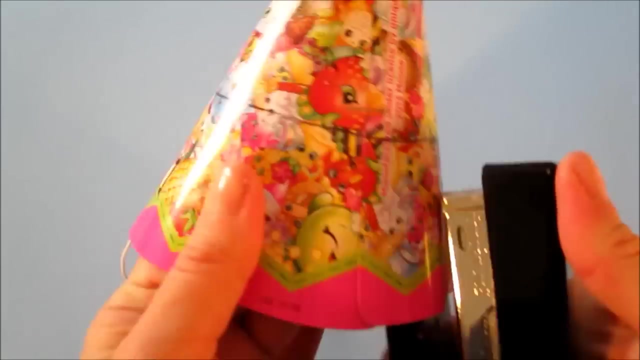 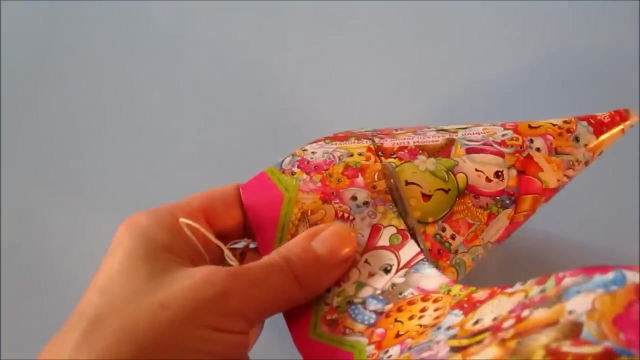 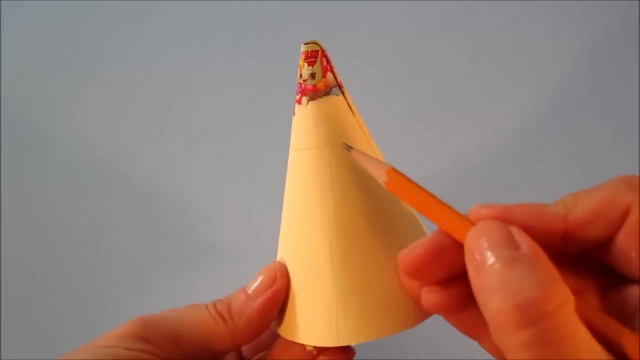 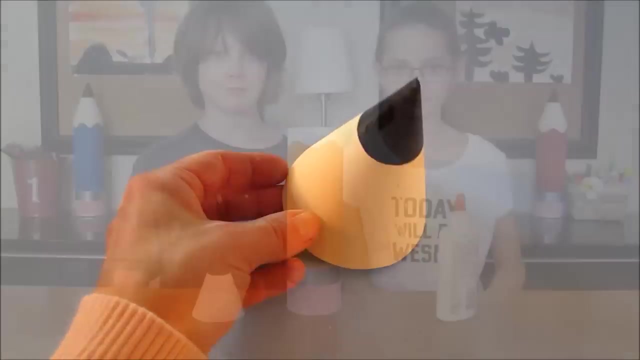 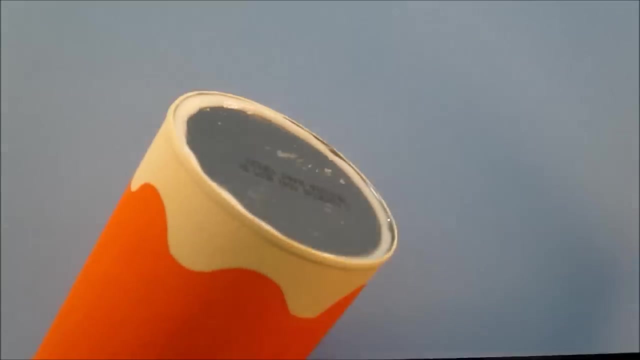 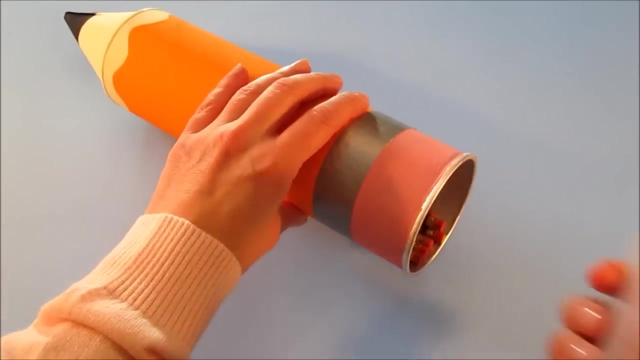 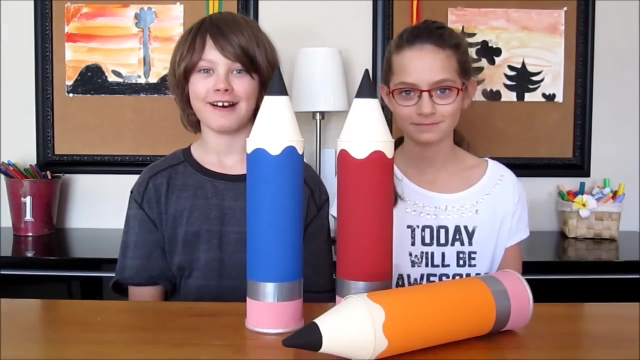 Thank you. Thank you, Thanks for watching and we'll see you next time. Bye, See ya.